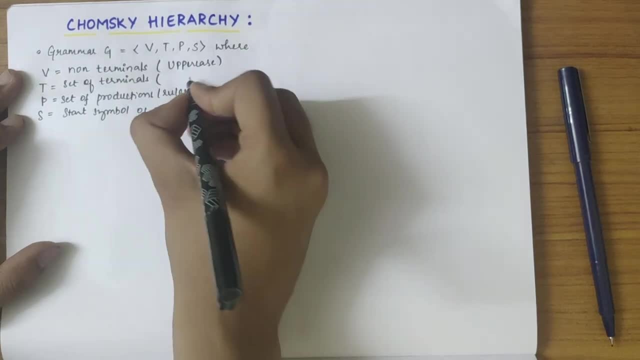 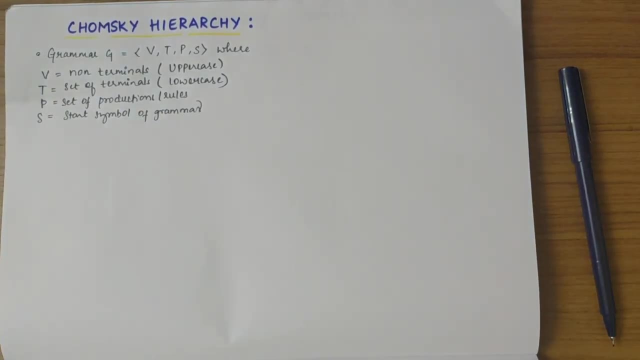 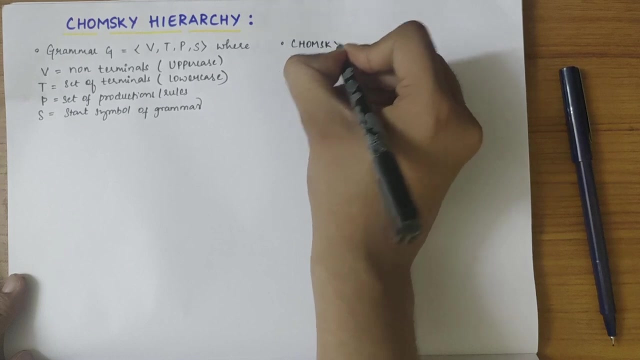 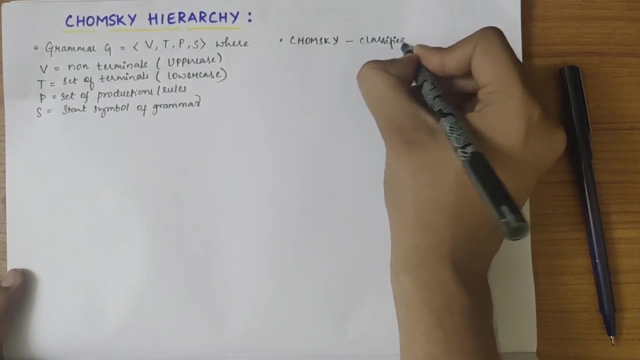 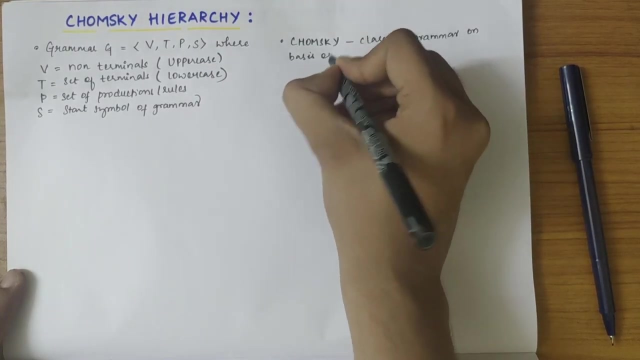 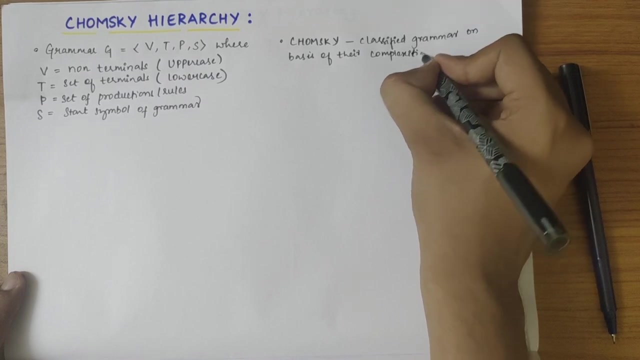 and the set of terminals are always in the lowercase. So with this basic understanding of grammar, now let's look into the classification. So Chomsky was an American scientist who classified the grammar on the basis of their complexities. So he classified the grammar into 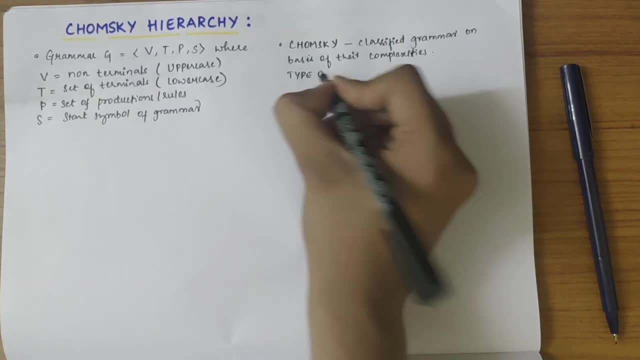 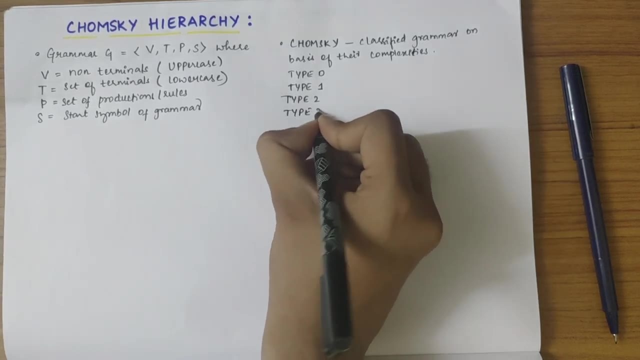 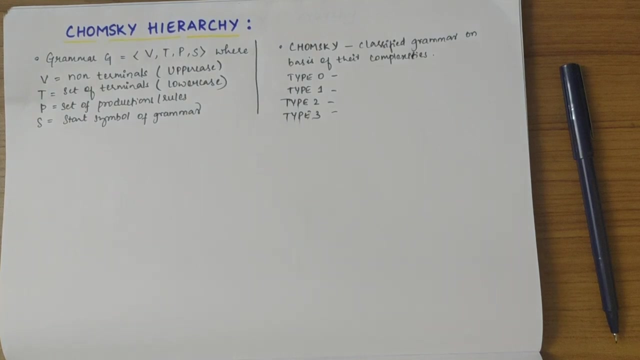 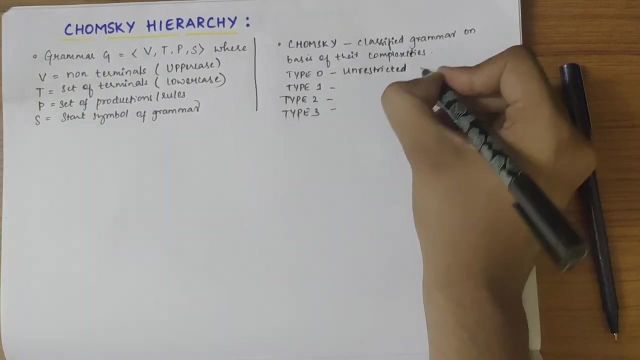 the following categories: Four types, that is, Type 0, Type 1,, Type 2, and Type 3.. So Type 0 grammar is also called as the unrestricted grammar. Type 1 is also called as the contracted grammar. 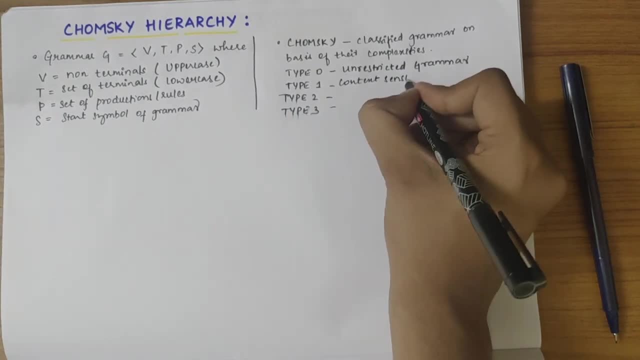 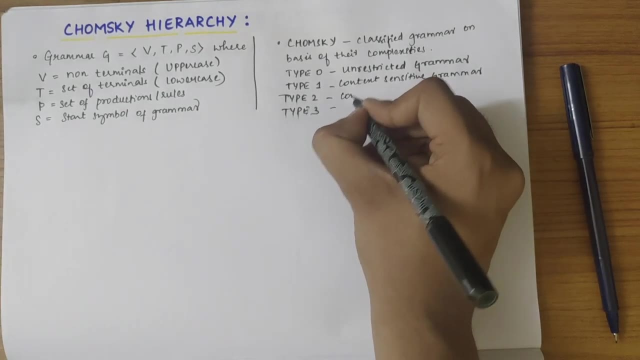 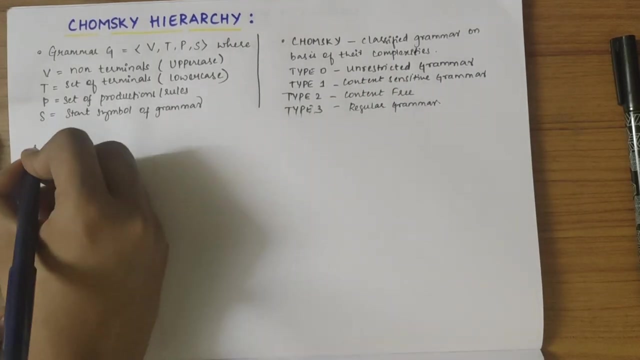 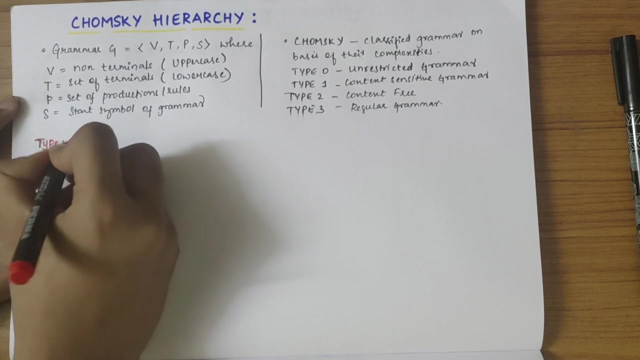 Type 2 is called as the context-sensitive grammar. Type 3 is the regular grammar. Now let's look into each type of grammar one by one. So first we have Type 0 grammar. So Type 0 grammar is also called as: 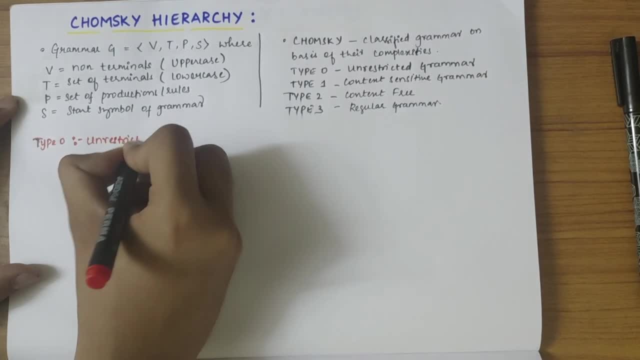 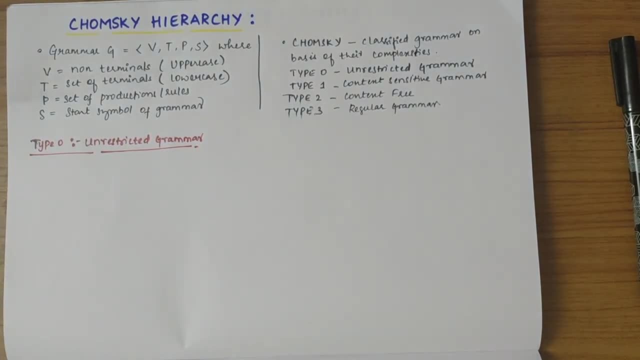 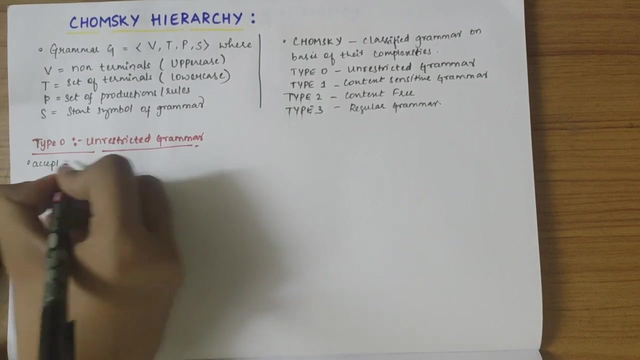 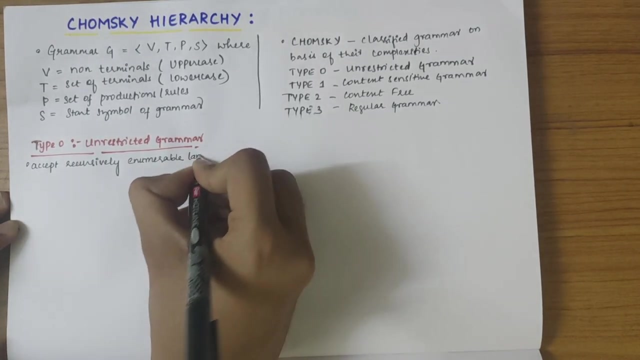 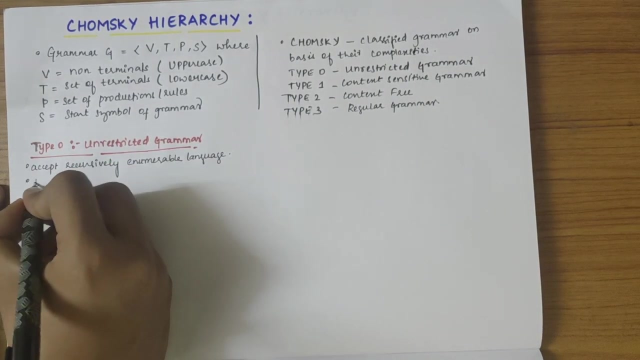 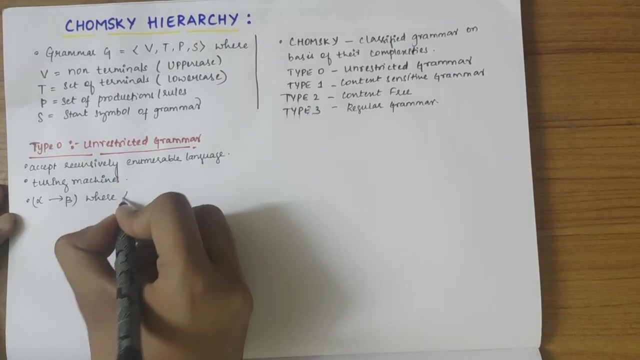 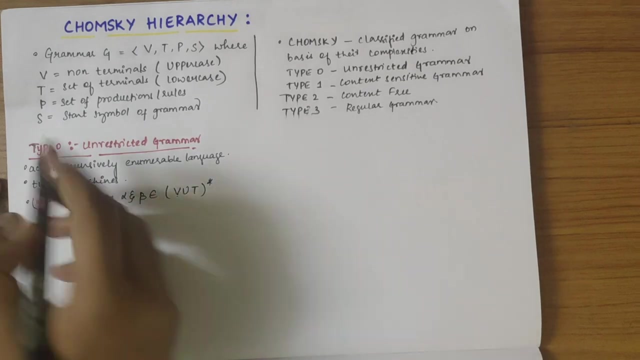 unrestricted grammar. So Type 0 grammar accepts recursively enumerable languages. So these languages are further accepted in the Turing machines. So here any grammar of the form alpha derives beta, where alpha and beta belongs to V union T star. here V is the non-terminals and T is the set of terminals. 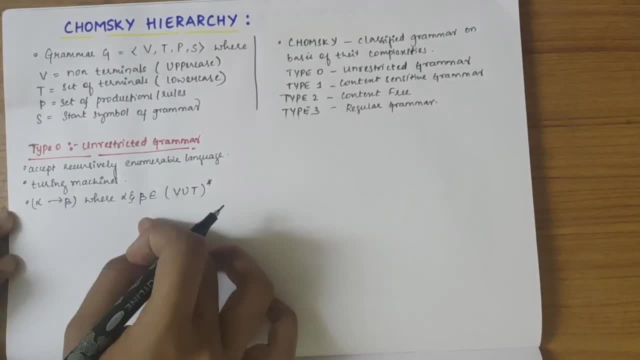 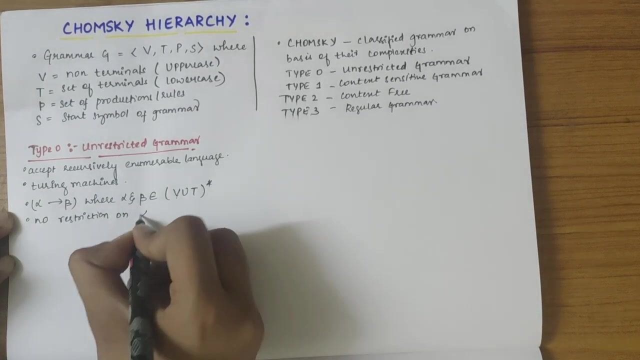 So here this: when the grammar is of this form, alpha derives beta. so here, in this condition, it is called as unrestricted grammar. So union of V, union T star. so here we need to understand that there is no restriction on alpha and beta. 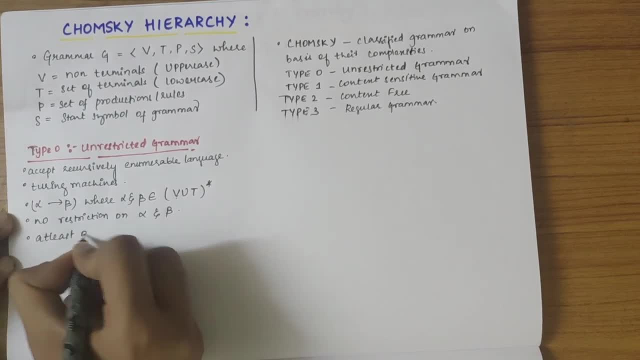 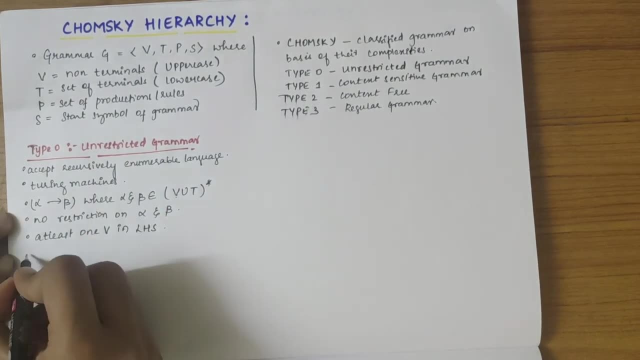 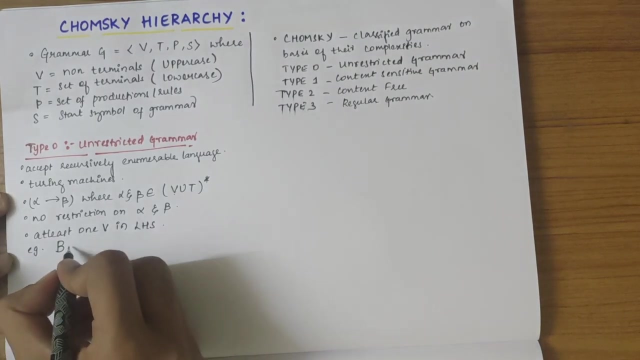 But one rule is that there has to be a term. There has to be at least one non-terminal in LHS side, that is in the alpha. So here, if you take an example like B, that is upper case non-terminal is there S and 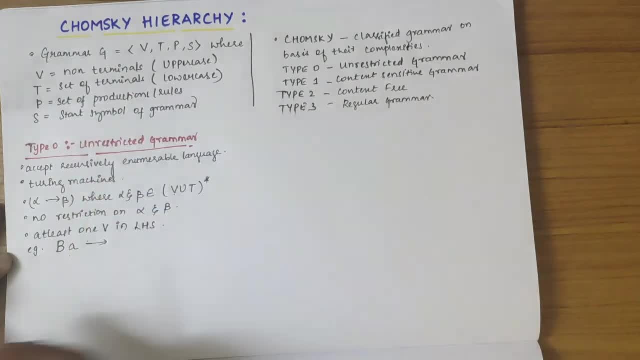 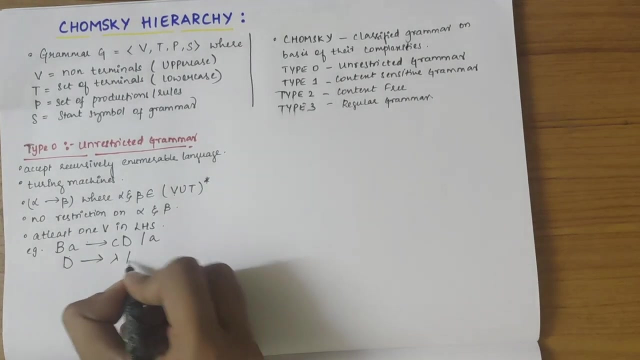 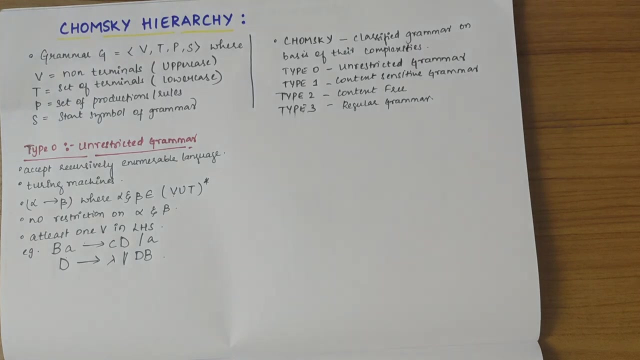 A followed by that. this is. this would be the set of terminals, lower case BA derives. here you can write C, D or anything, or it could be just a single non-terminal. Non-terminal derives lambda or DB or anything. So this is type 0 grammar. 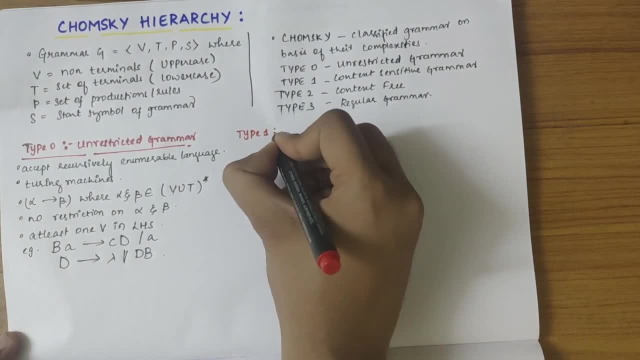 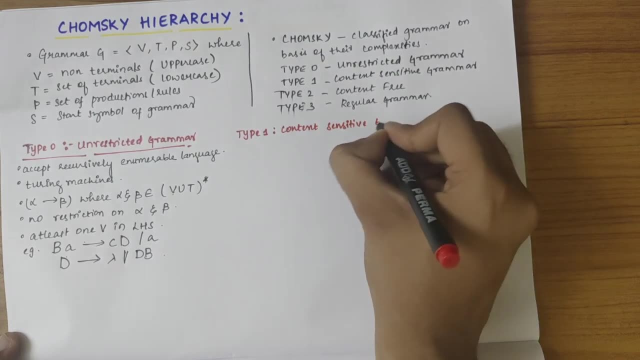 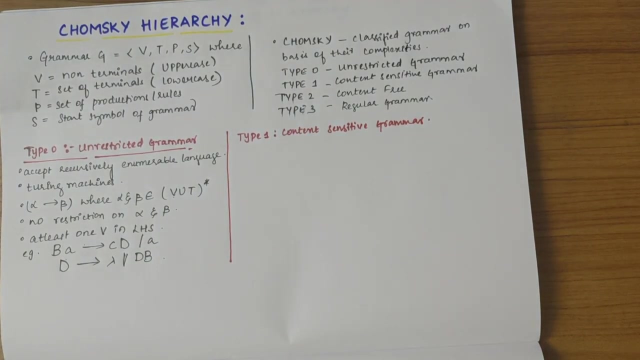 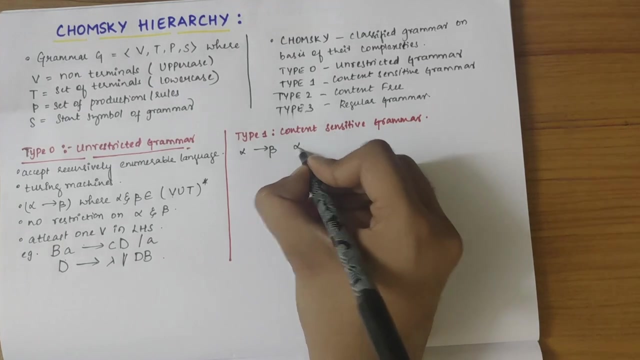 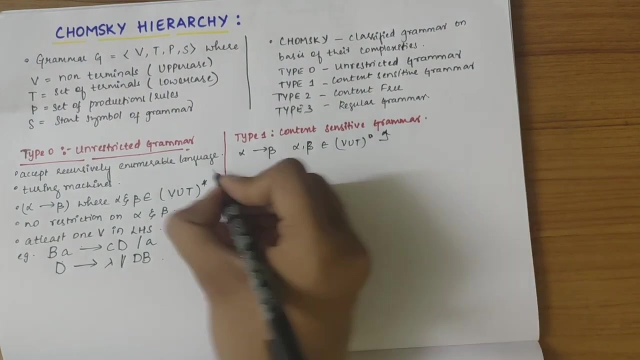 Now let us look into type 1 grammar. that is also called as context sensitive grammar. So any production, Any production that belongs of the form alpha derives beta, such that alpha and beta belongs to V union T star, is called as context sensitive grammar. 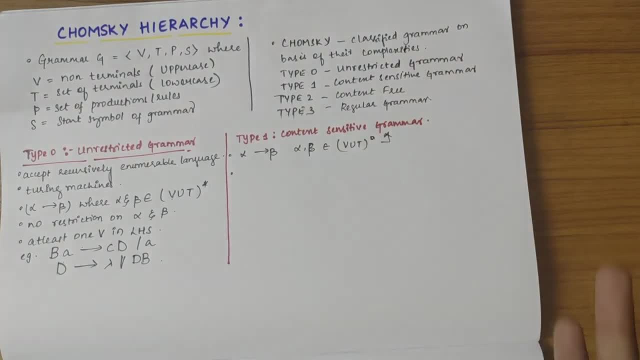 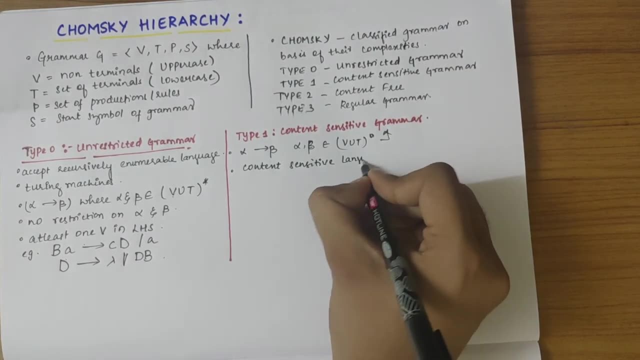 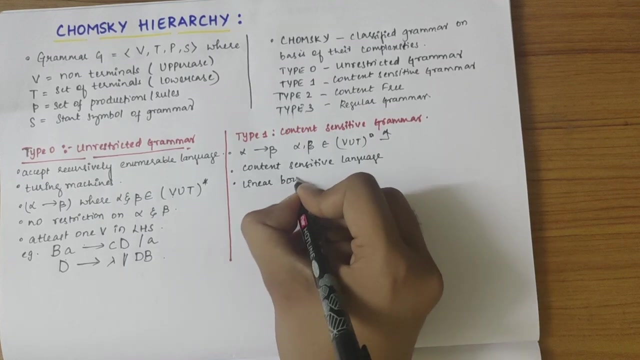 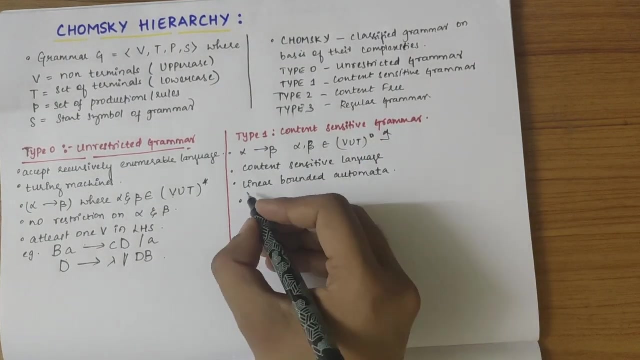 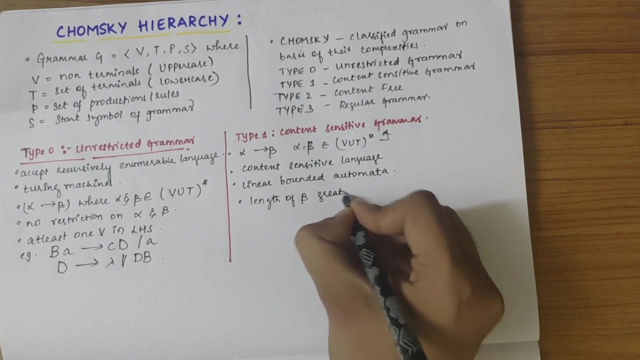 So here any language which obeys the context sensitive grammar is called as context sensitive language. So this language is accepted or used in the context sensitive grammar Linear bounded automata. So here we have one restriction, that is, the length of beta should be greater than greater. 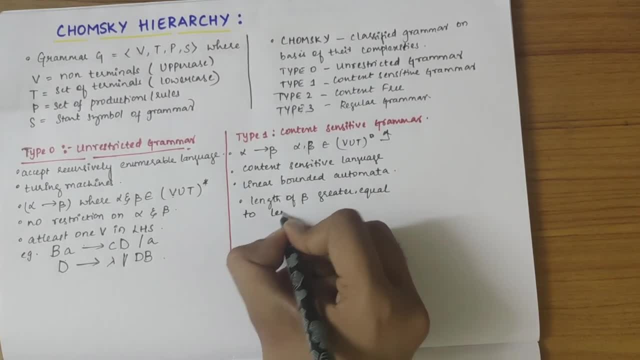 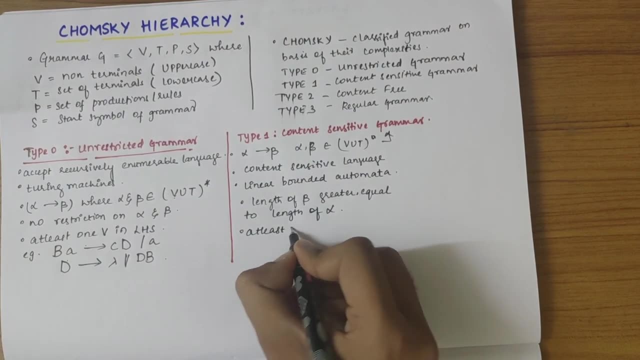 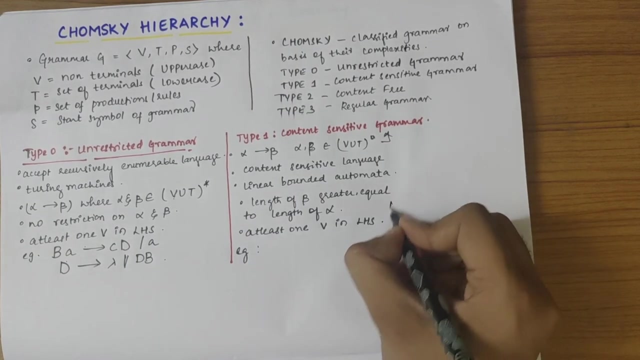 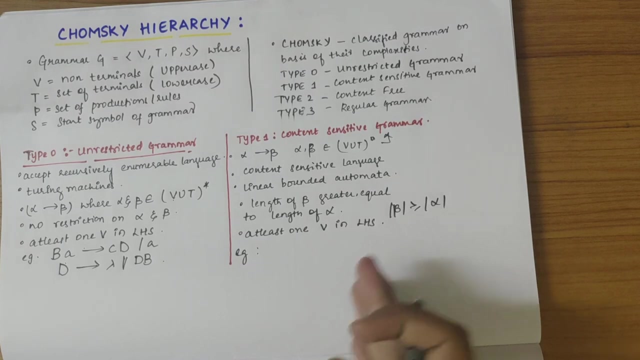 or equal to length of alpha, And there has to be at least one non-terminal in LHS. The other one is the length of alpha. So we are considering this kind of combination and we have to consider each one in next side. so considering an example. so here, beta, mod of beta, that is mod of beta like the length of. 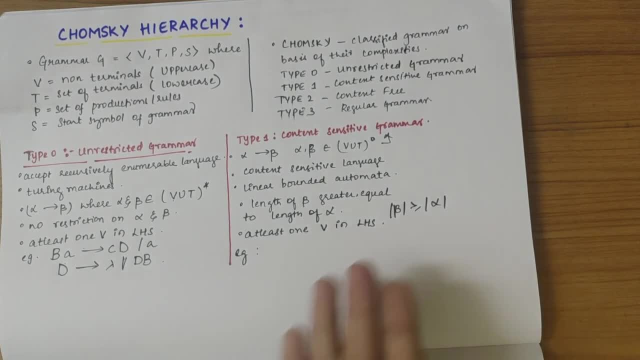 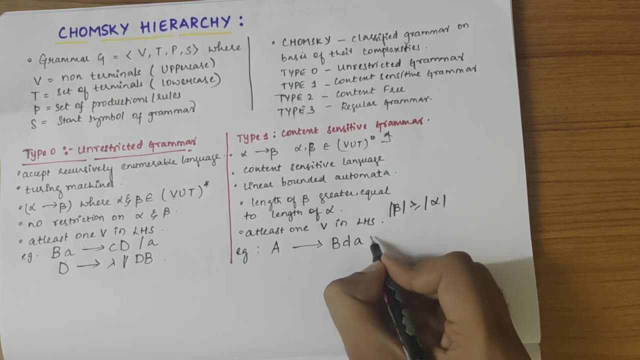 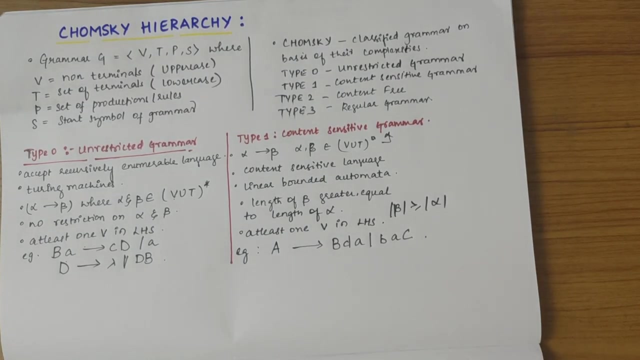 the length of beta should be greater than the length of alpha. this is the basic condition of context sensitive grammar. so if you look at an example, a derives b, d, a, b a c. so here the length of beta is greater than length of a right. so yes, or we can take another example: a derives 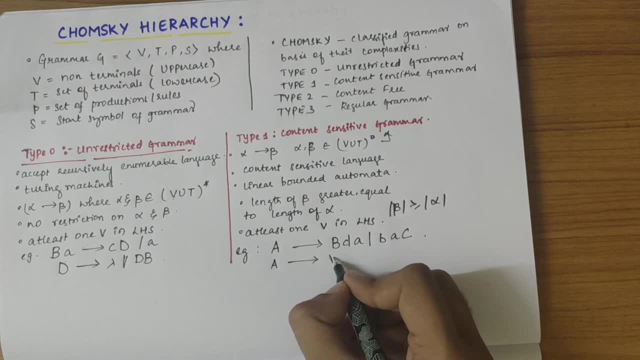 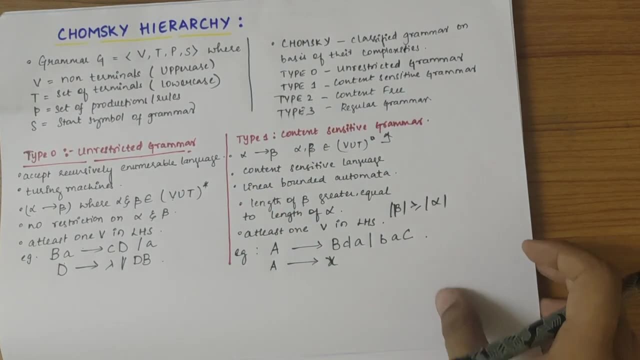 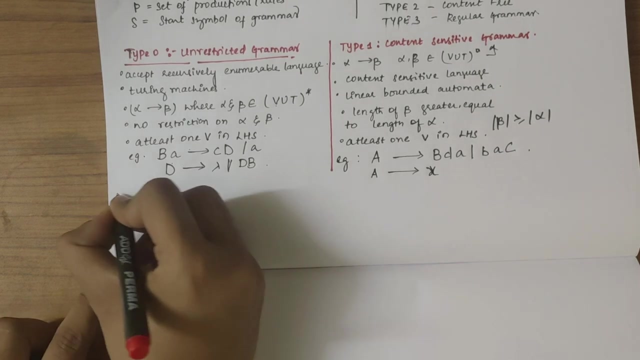 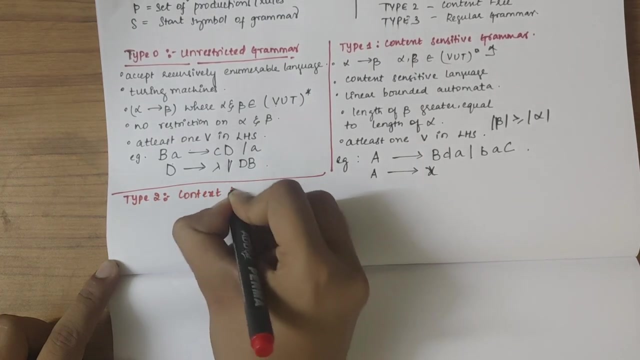 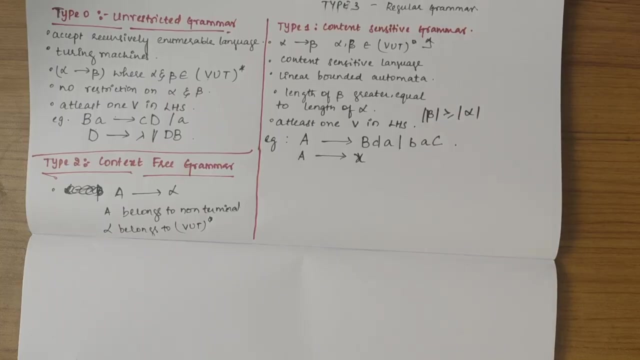 let's write x, okay, so the length is equal. so in this case also, it is context sensitive grammar. so now let's look into the type 2 that is context free grammar- context free grammar. now let's look into the type 2 that has context free grammar. any production of 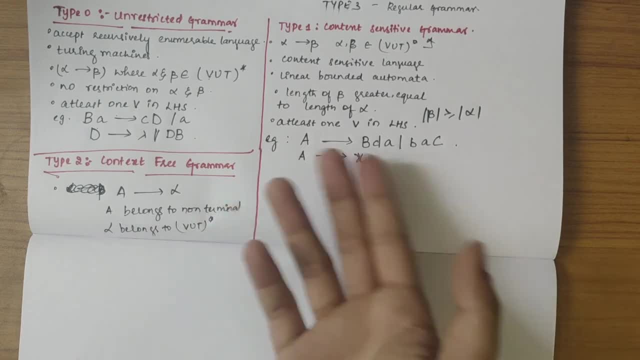 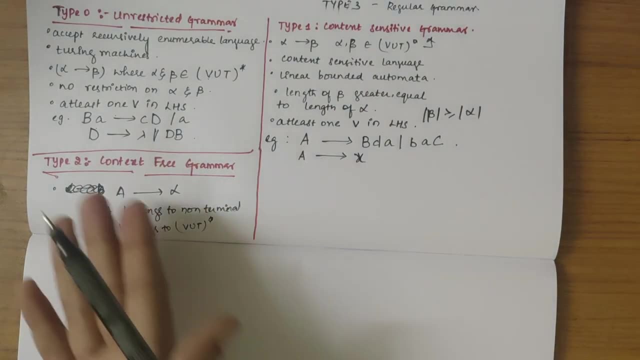 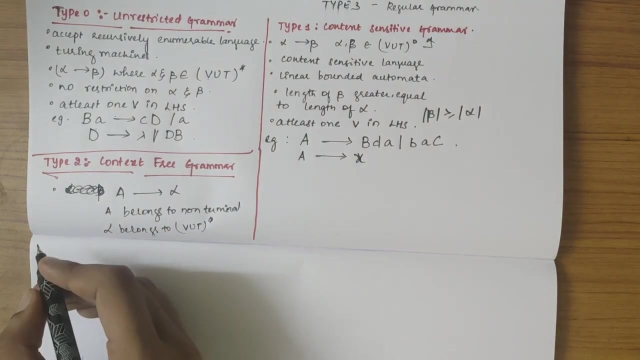 the form a derives alpha, where a belongs to the non-terminal, that is v, and alpha belongs to v, union e star, so is said to be the context free grammar, and any language obeying this is called as context of free language. so here this context free language is used in pushdown automata. 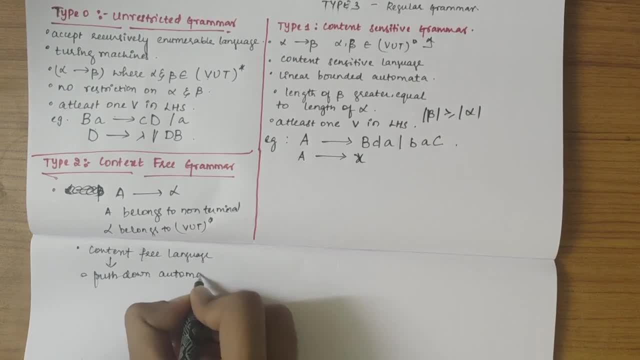 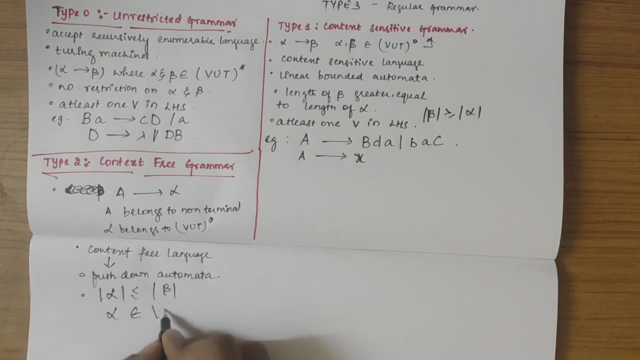 so here we have condition, that is, mod of alpha should be less than mod of beta, that is, the length of alpha should be less than or equal to mod of beta, and alpha should belong to the v. yes, we have seen, and along with that we have mod of alpha should be equal to 1. so on lhs, it has to be. 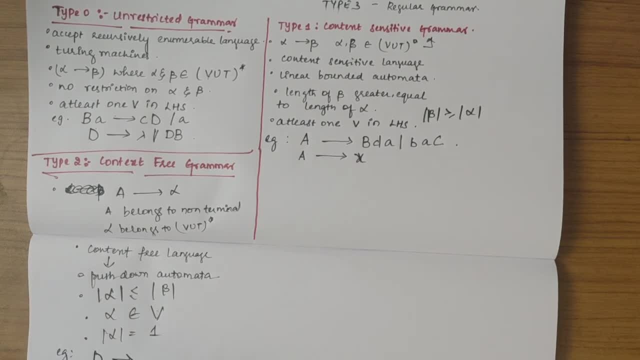 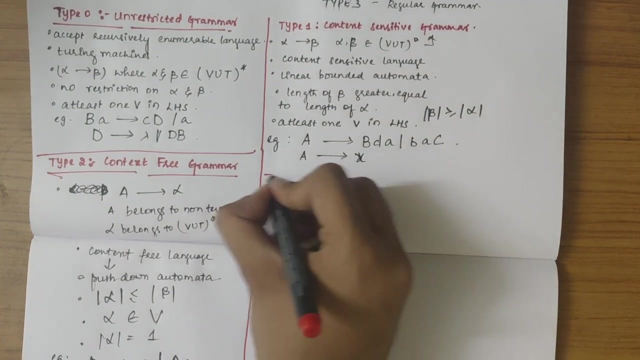 always 1. so let's look into an example that is d derives alpha, or a a, or it could be a derives a c or anything. so this is type 2, that is context free grammar. now looking into the type 3, that is the regular grammar. 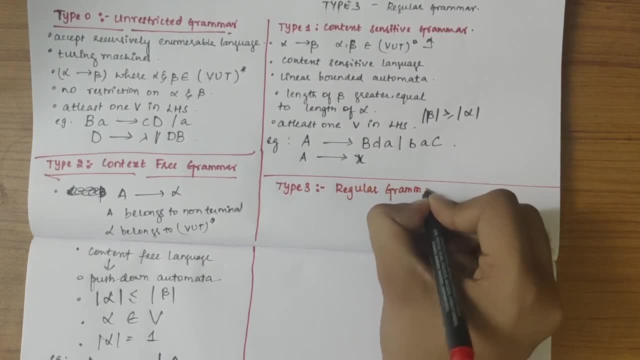 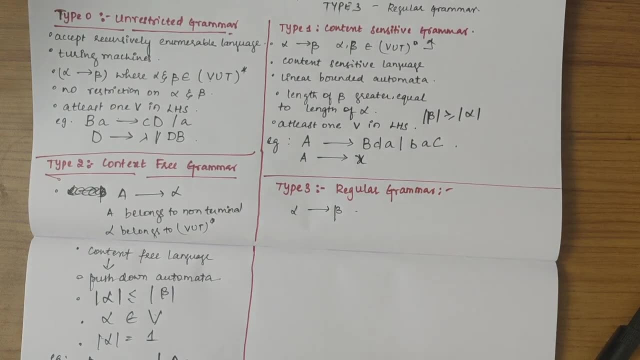 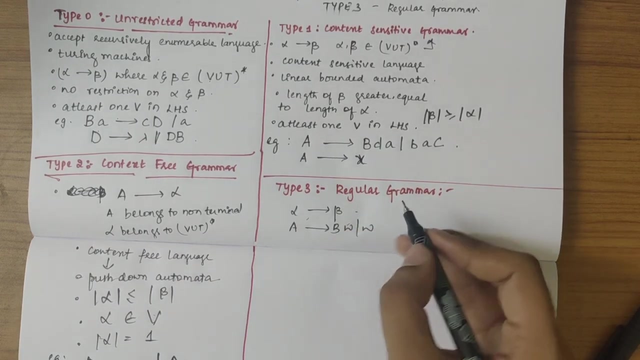 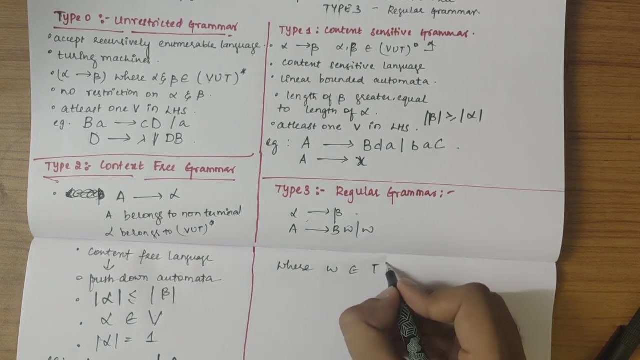 so any production of the form Alfa- there is beta, or here let's take a- derives b, b, w, w, where w belongs to B w, where w belongs to is to t star, that is the terminal set of terminals, and a? b belongs toермinal set of terminals and a b long belongs to there. tonal s & i. 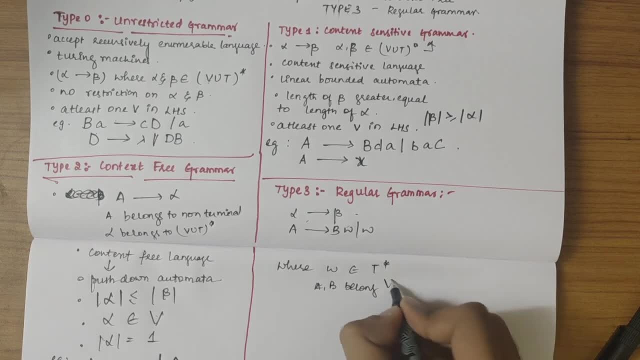 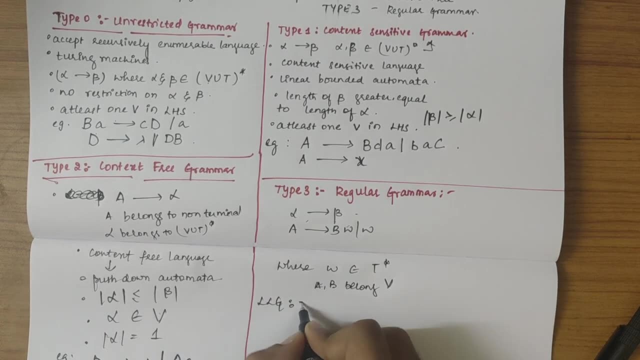 stand here n Sonic. So to the v, that is, the non-terminals, is said to be left linear grammar. So for left linear grammar we have the condition as a derives b, w, w. So here a non-terminal is followed by the terminal. 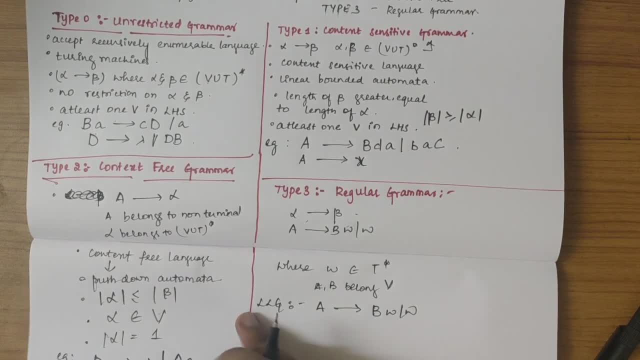 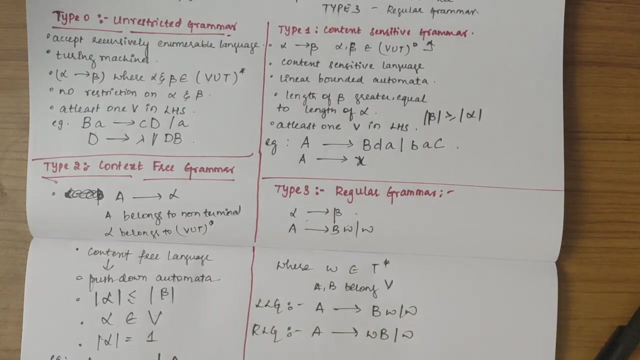 right. So looking into the this was left linear grammar, looking into the right linear grammar, we can write it as a derives w, b, w. So here a non-terminal is here. So here a terminal is followed by the non-terminal. So this is the right linear grammar, So this type of grammar. 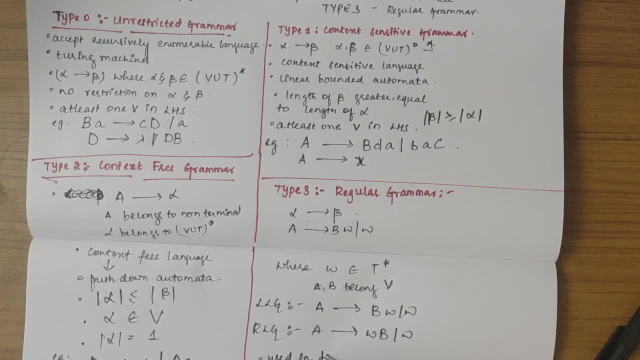 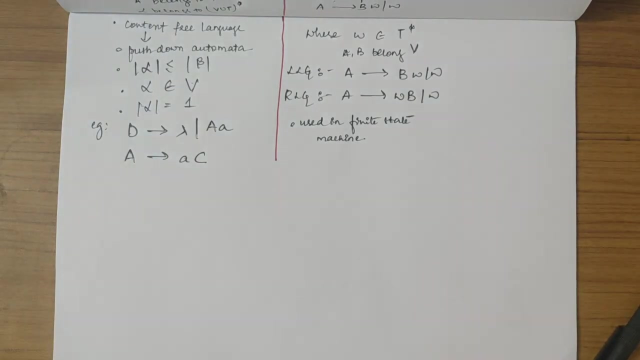 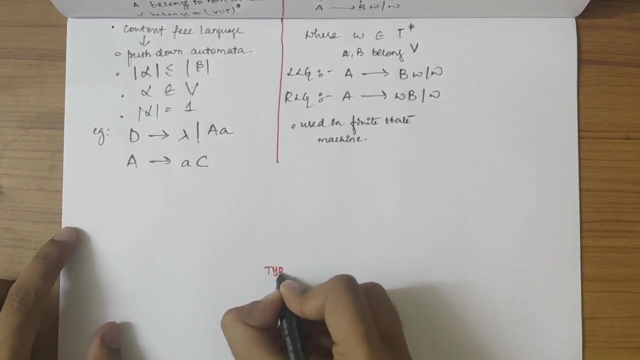 is used in the finite state machine. So this was about the regular grammar. This was about the regular grammar. So here you can broadly classify or conclude the types of grammar with a diagram. that is we. first we have type 0, that is the no. let's start from the type 3, that is regular grammar. Then we have the type 2. 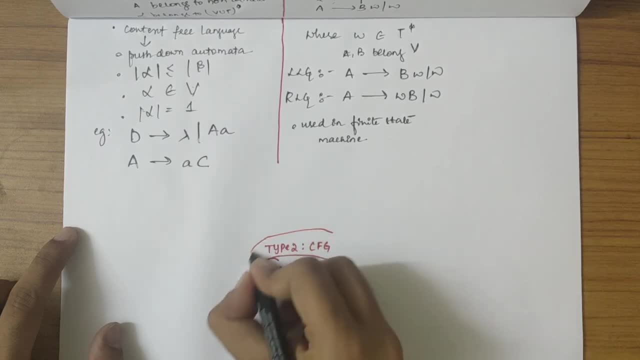 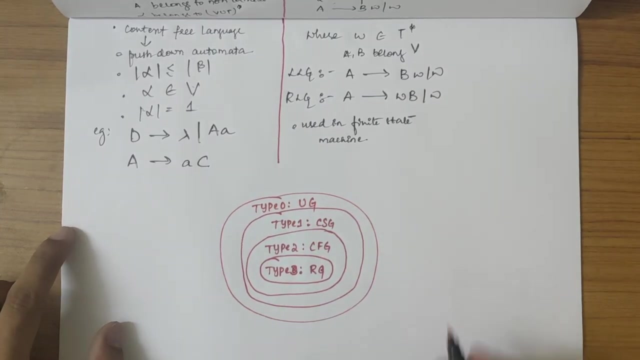 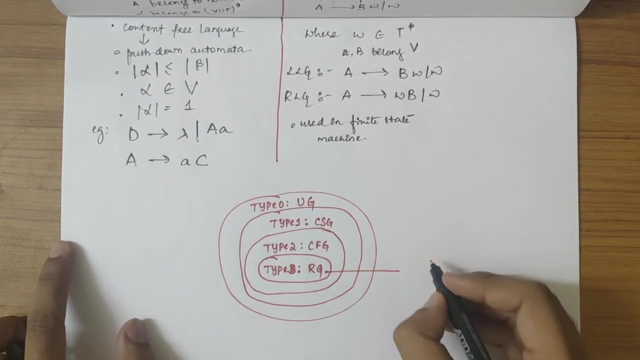 that is the context-free grammar, followed by that we have the type 1, that is context-sensitive grammar. Then we have the type 0, that is the unrestricted grammar. So here these grammarers are being used, or the regular grammar is used in finite state machines.